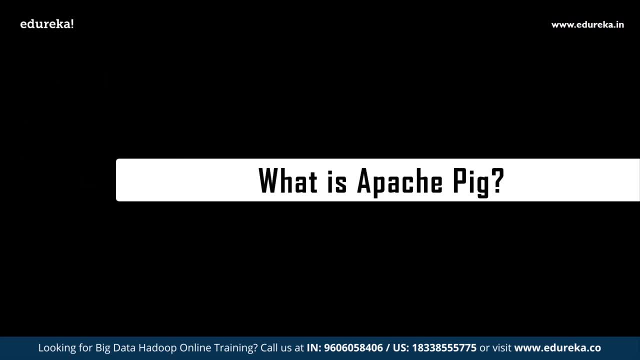 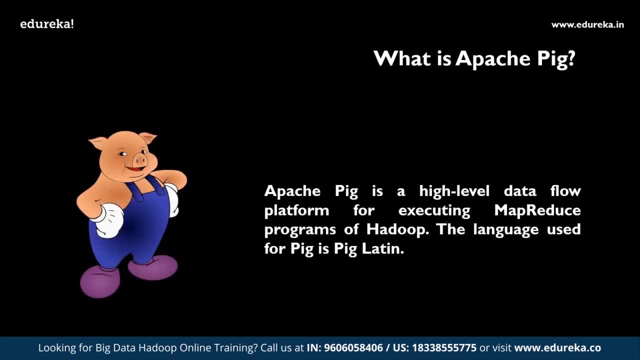 So the first one is: what is Apache pig? So Apache pig is an abstraction over MapReduce. It is a tool or platform which is used to analyze larger sets of data, representing them as data flows. Pig is generally used with Hadoop. We can perform all the data manipulation operations in Hadoop. 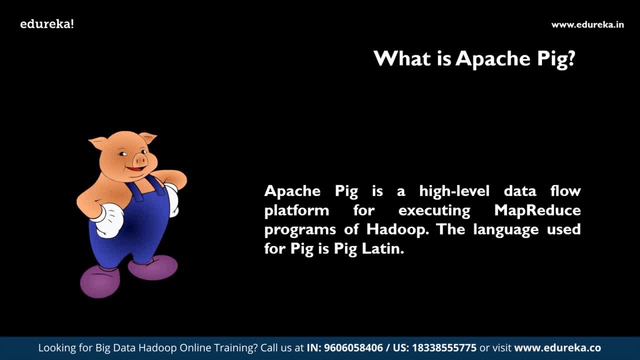 using Apache pig. To write data analysis programs, pig provides a high-level language known as pig Latin. This language provides these operators using which programmers can develop their own functions for reading, writing and processing data. To analyze data using Apache pig, programmers need to write scripts using pig Latin language. 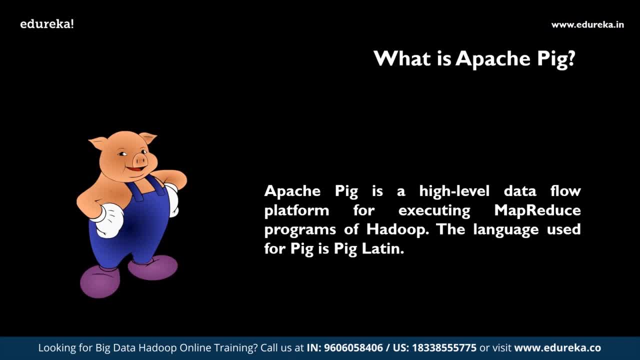 All these scripts are internally converted into map and reduced as, respectively. Apache pig has a component called Apache pig engine that accepts the pig Latin scripts as input and converts those particular scripts into MapReduce jobs. So this was the basic introduction to Apache pig. Now moving ahead. 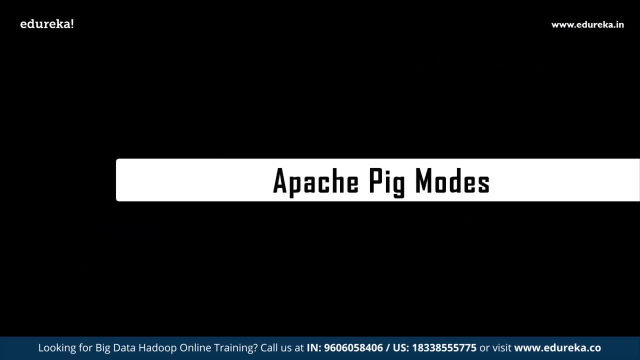 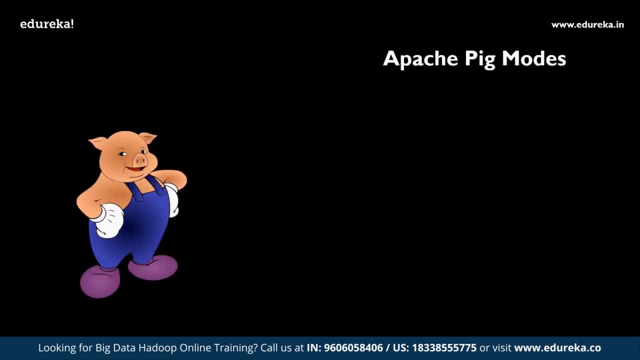 we shall understand the different modes in which Apache pig functions. There are two particular modes in which Apache pig functions. Those are the local mode and MapReduce mode. First we will understand what exactly is local mode. In local mode, Apache pig is designed to execute in a single JVM. 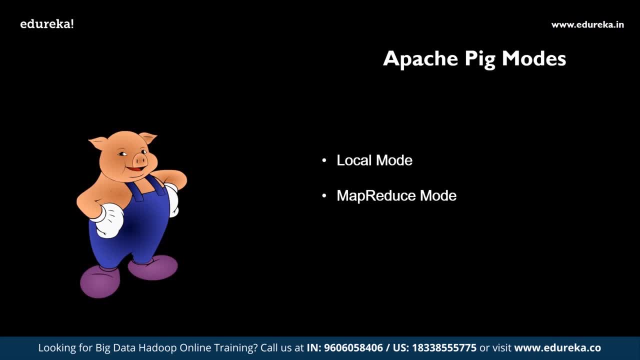 and is used for development, experimenting and prototyping. Here files are installed and run using localhost. The local mode works on local file system and the input and the output data is stored in the local file system. To access the command or the crunch shell in local mode: 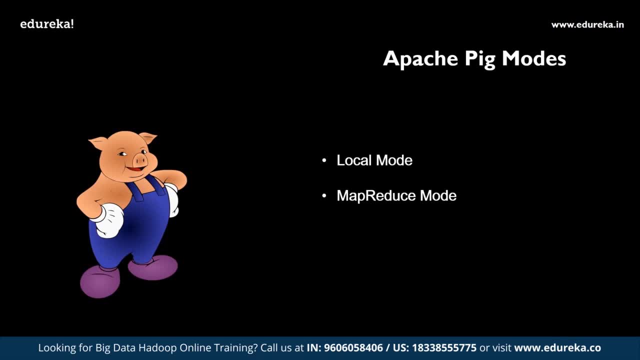 you need to execute a command called pig-x local. We shall practically execute this in the demo section. Now, moving ahead, we shall discuss about the second type of mode in which Apache pig can be run, That is, the MapReduce mode. The MapReduce mode is also known as Hadoop mode. 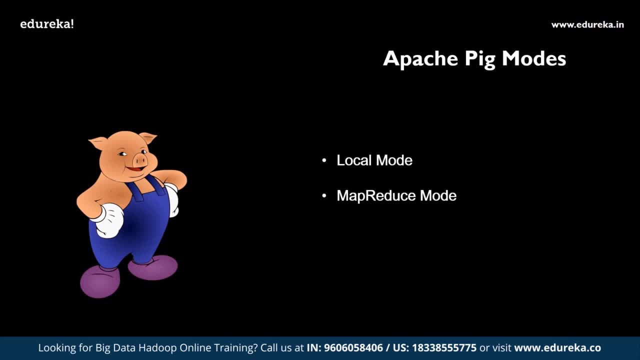 Apache pig chooses Hadoop mode as its default mode In this pig renders pig Latin into MapReduce jobs and executes them on a Hadoop cluster. It can be executed against semi-distributed or fully distributed Hadoop installation. Here the input and the output are present on HDFS. 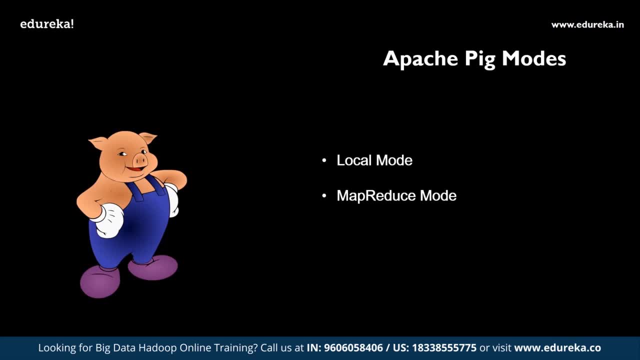 The command for executing pig in MapReduce mode is pig or pig-x MapReduce. Again, we shall discuss about this particular command in our demo section, where I'll show you both the modes and execute the pig scripts there Now, followed by the pig modes. 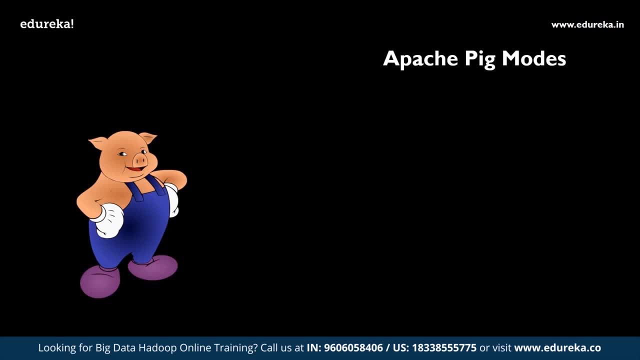 we shall understand the ways to execute pig program. So basically, the pig scripts are executed in three parts, In particular modes. those are interactive mode, batch mode and lastly, the embedded mode. Don't worry, I'll explain to you each of these modes. 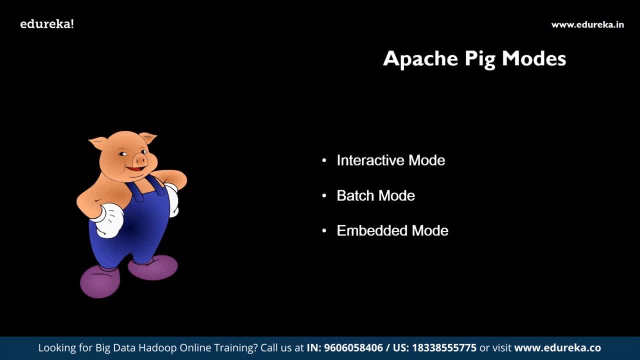 Firstly, we shall discuss about the interactive mode. In this particular mode the pig is executed in a grunt shell. To invoke grunt shell, run the pig command. Once the grunt mode executes, we can provide pig Latin statements and command interactively at the command line itself. 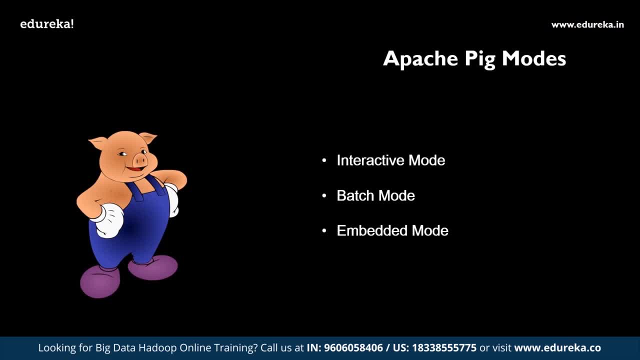 So the next mode is the batch mode. In this particular mode we can run a script file having a dot pig extension. These files contain the pig Latin commands. So basically what we do is we write the pig command or the pig script and store it in a location. 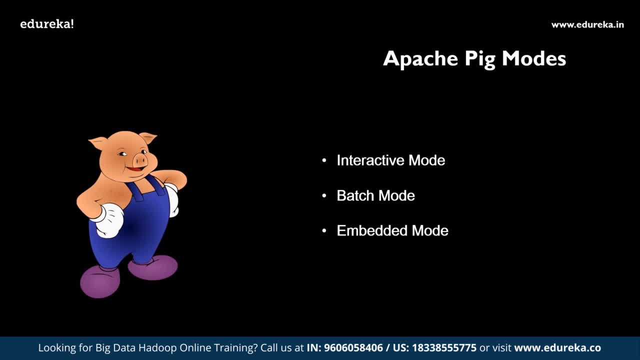 And using the terminal, we will access that particular location and that particular file and run the code present in that file. So this is what happens in batch mode. So, followed by that, the last mode is the embedded mode In this particular mode. 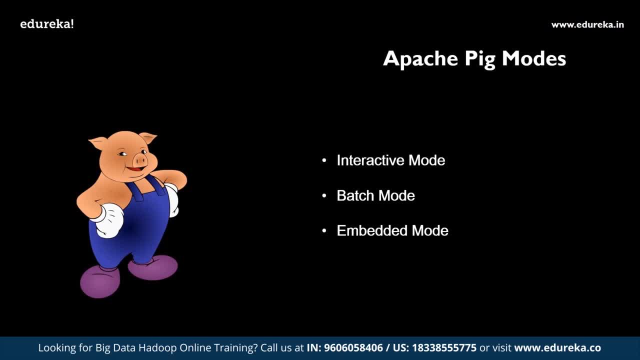 we can define our own functions. These functions can be called as user-defined functions. Here we use programming languages like Java and Python to define our own user-defined functions. So these were the three different modes in which we can execute pig scripts. Now moving ahead. 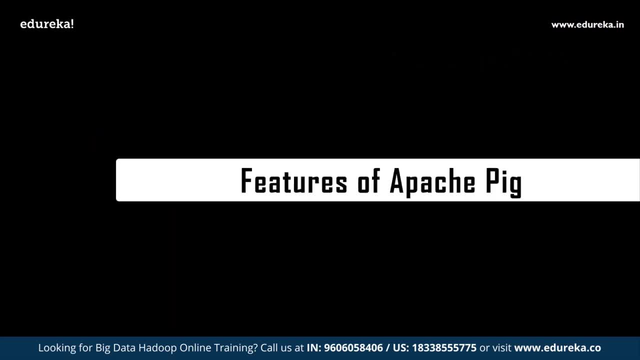 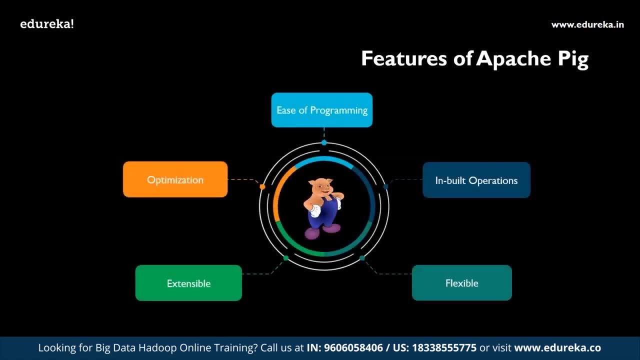 we shall enter into our next topic, that is, the features of pig. So there are five different modes and important features of pig. So first up, we shall understand the ease of programming. Writing complex Java programs for MapReduce is quite tough for non-programmers. 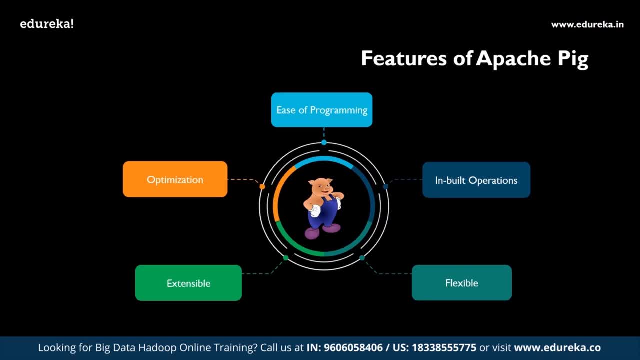 Pig makes this process very easy. In the pig the queries are converted into MapReduce processes internally, So obviously it has grown the ease of programming. Followed by that. the next important feature is the optimization opportunities. So what exactly is optimization? 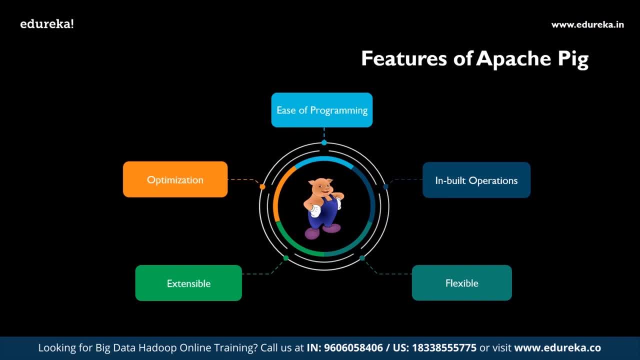 It is how the tasks are encoded- permits the system to optimize the execution automatically, allowing the user to focus on semantics rather than efficiency. So, followed by the optimization, we have the extensibility: A user-defined function is written in which the user can write their logic. 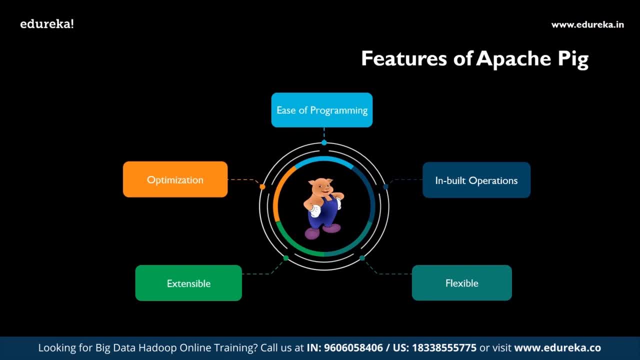 to execute over the data sets, So this increases the extensibility of the programmer. Followed by that, the next important feature is it is highly flexible. Apache Pig can easily handle structured as well as unstructured data, So Apache Pig tool is considered to be highly flexible. 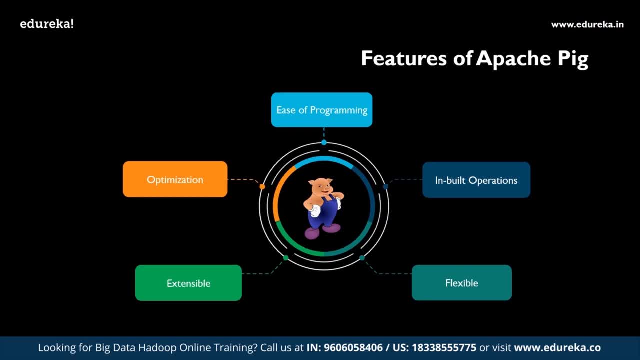 irrelevant of the data type. Followed by that, the last and important feature is inbuilt operators. Apache Pig contains various types of operators, such as sort, filter, joints and many more, which are inbuilt. So here the programmer doesn't have to program. 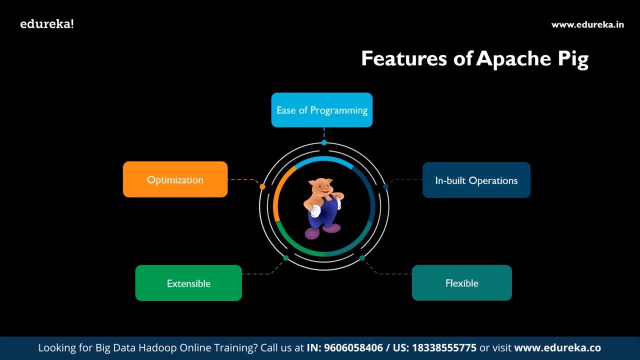 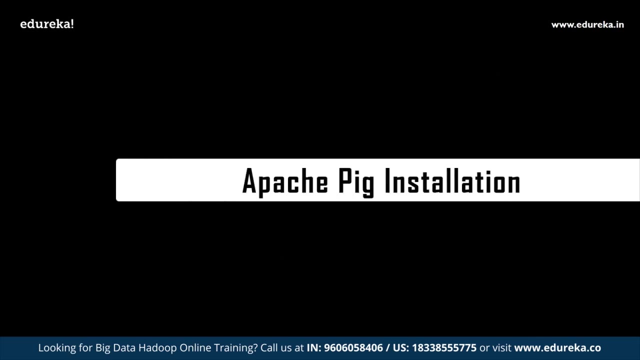 these functions externally. Instead, he can just directly get an access to those inbuilt functions and execute them. So these were the five important features of Apache Pig. So the next topic in our today's discussion is Apache Pig installation into our local system. 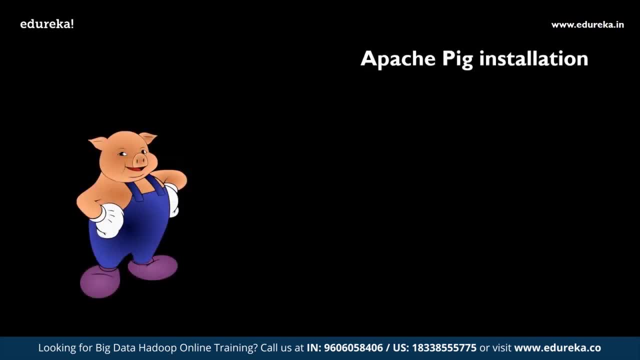 Now we shall discuss about one of the easiest ways to install Apache Pig into our local system. So today I'll explain you how to install Apache Pig into Windows operating system. So to do this, the easiest way is to download one of the virtual machines. 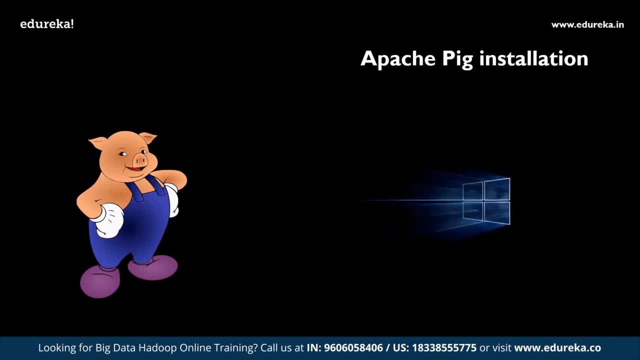 So I would prefer you to download Oracle VirtualBox for this particular task. Followed by that, we shall also download a quick start VM of CloudARAM. Don't worry about the softwares. I'll drop down the link for those softwares in the description box below. 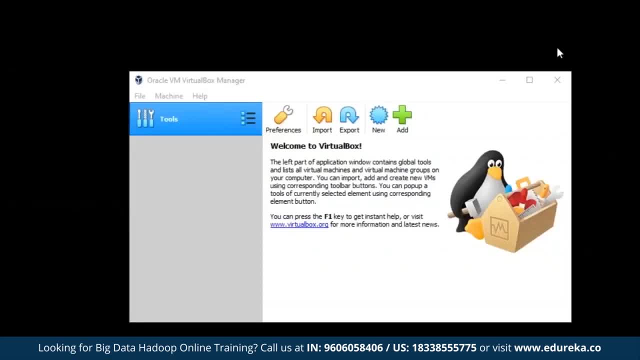 You can use that and download them. So, once after the Oracle VirtualBox is installed into a local system and it is running, this is how it looks like. Now what we want to do is to add a new virtual machine into our virtual box. 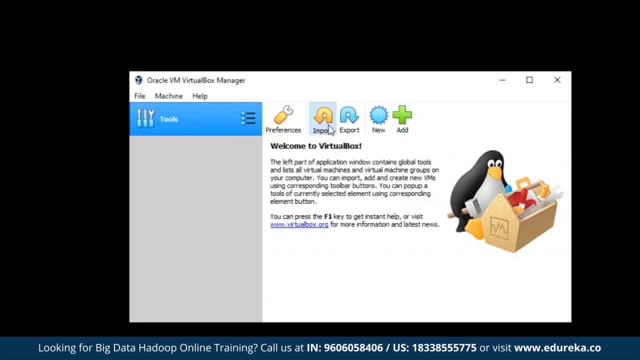 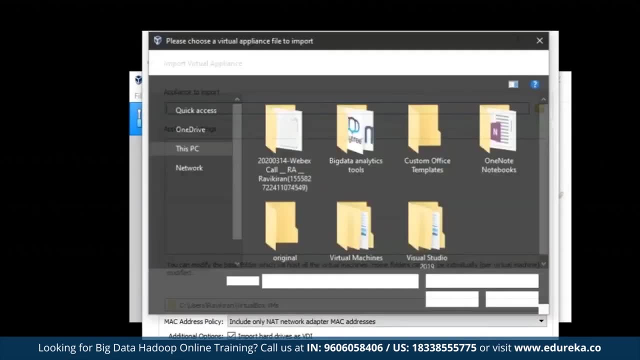 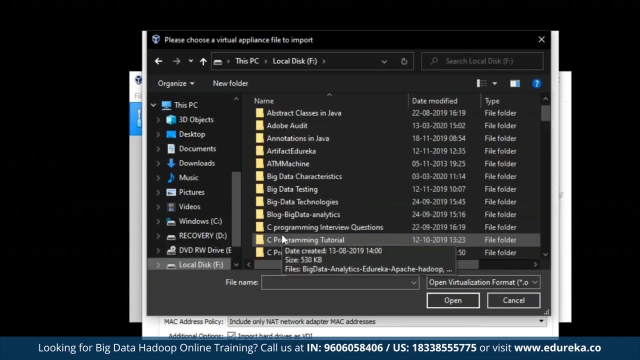 So for that you just need to select import option and it will give you a new dialog box And from here you must redirect to the location where your virtual box is located. So in my system it's located in F drive And inside F drive. 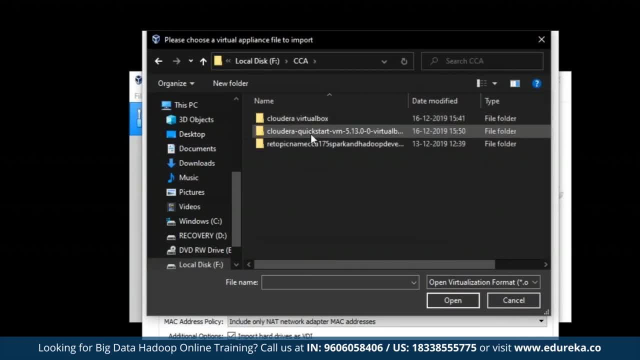 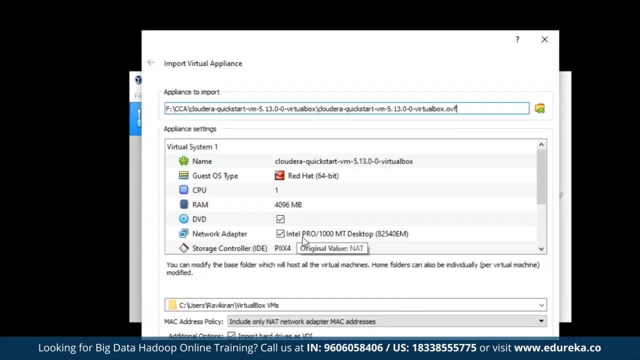 CCA CloudARAM VirtualBox, CloudARAM Quick Start VM. So there you go. Now you just have to select open, And before we actually select the button import, you might want to select the RAM and increase its size to at least 8 GB. 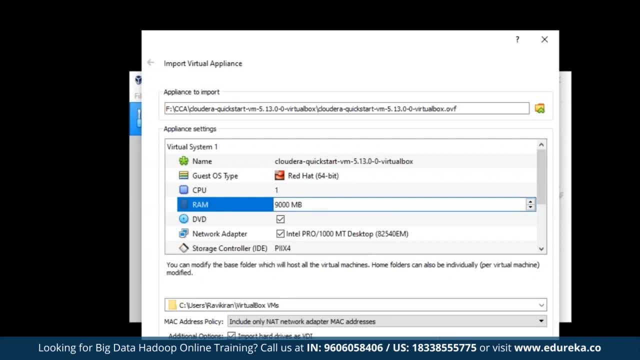 So just write in 9000 MB, which is just a little about 8 GB. Now we are good to go. Just select the option import and your virtual box will be imported. You can see that the Quick Start VM is getting imported. 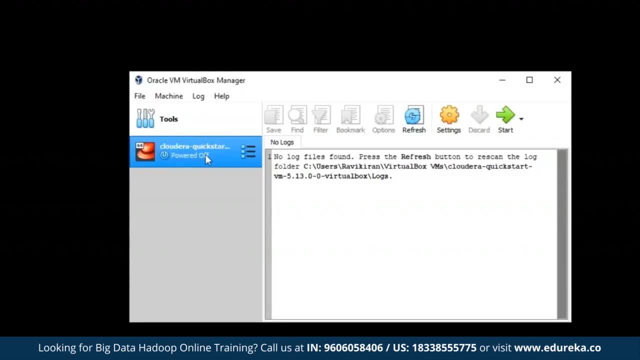 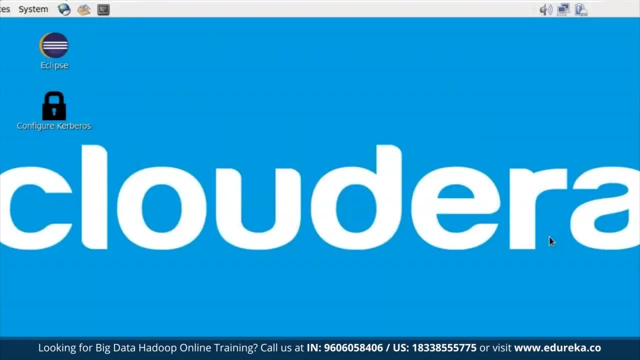 Now you can see that the virtual machine got successfully imported. Now to start it, all you need to do is just click on it and then select the start button, So you can see that the CloudARAM Quick Start VM version 5.13.0. 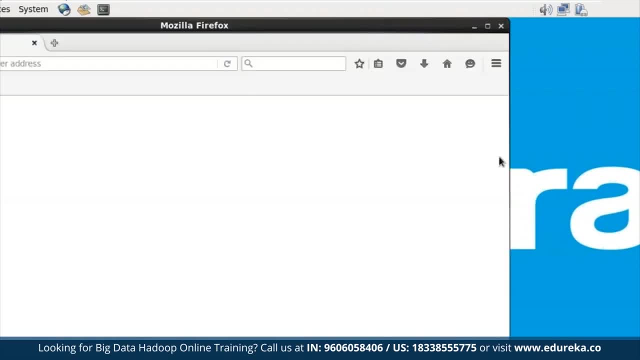 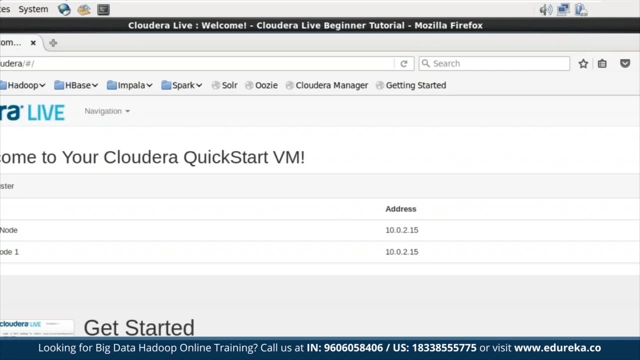 has been successfully imported and booted up. Here we are. We have the Quick Start CloudARAM VM. welcome note. And now, if you want to start up with a big editor, you might want to log into Hue first, or your HDFS, Remember, in CloudARAM. 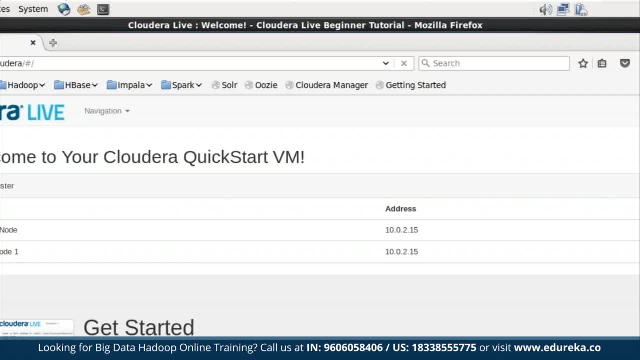 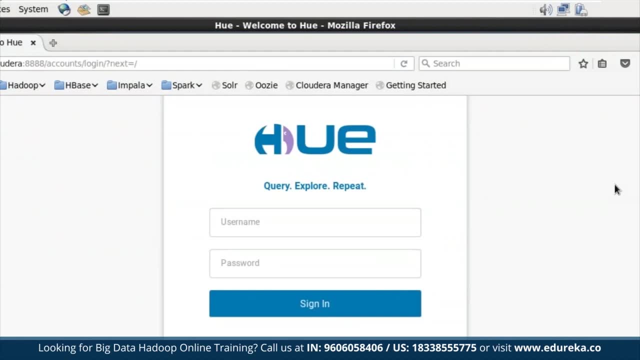 the default username is CloudARAM and the password also is CloudARAM. Now let me tell you: in CloudARAM, the default username and password for everything is CloudARAM. For example, let's log into our Hue using the username CloudARAM and password: CloudARAM. 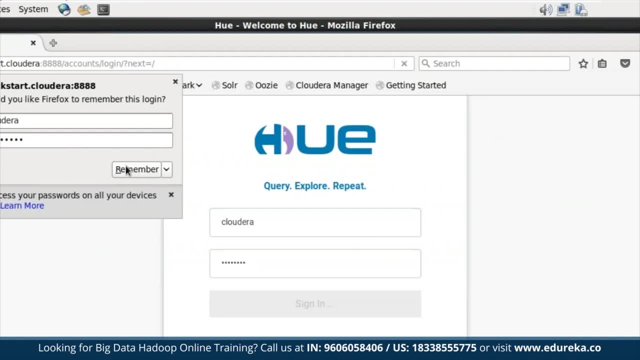 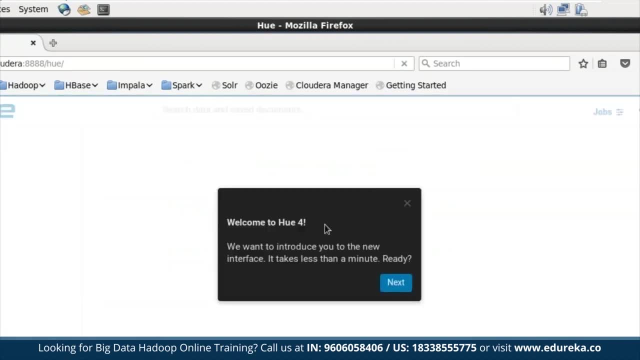 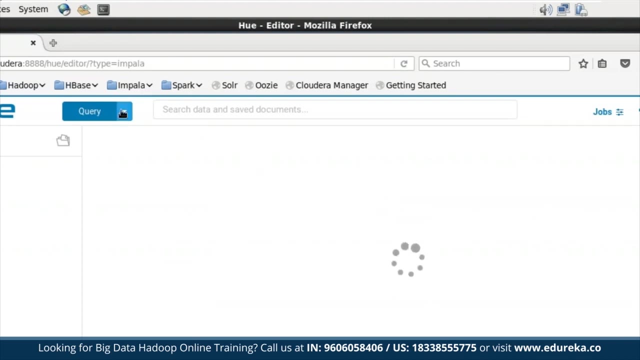 Now you might want to just select remember to remember your password. And there you go. You have successfully logged into Hue. And now, if you want your query editor for PIC, you can just select the bottom arrow mark and there you can select editor. 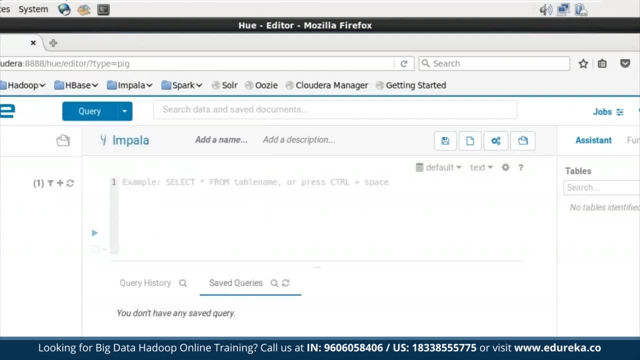 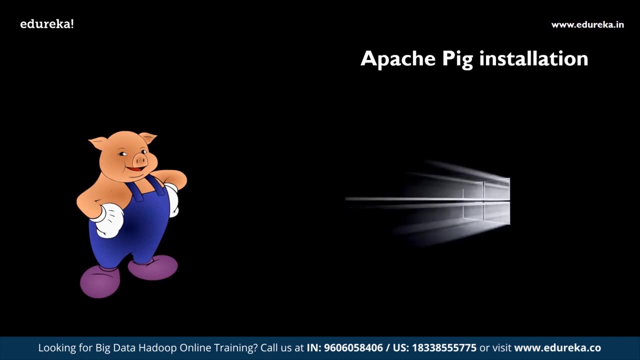 And inside editor you have the editor designed for PIC. Now you are in the window where you can write PIC scripts and execute them. Now we will move ahead into our next topic And, after finishing the theory part, we shall come back into our cloud era. 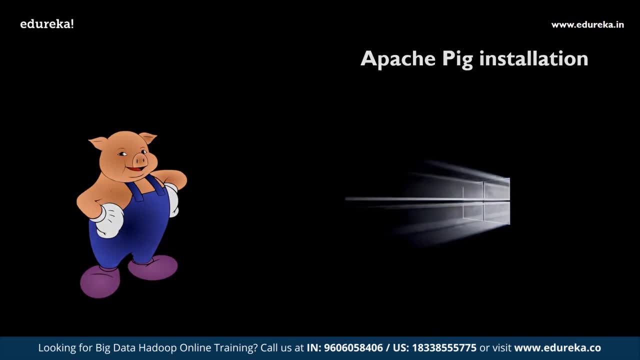 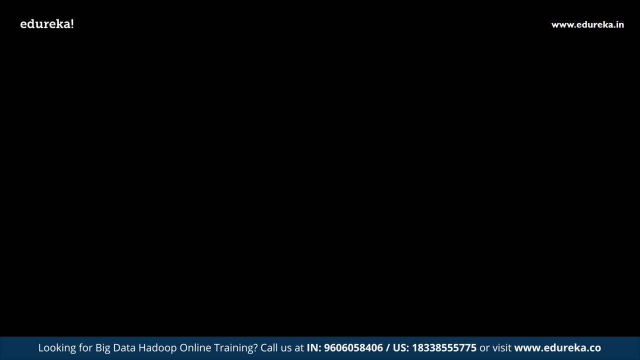 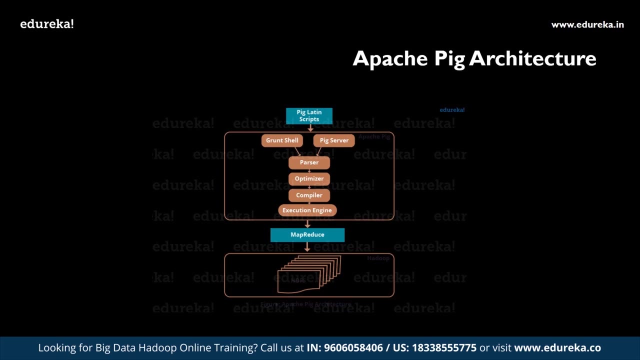 and execute some of the basic operations on PIC terminal. So our next concept is understanding the PIC architecture. So first of all let us go through the diagram of PIC architecture. The following diagram represents the architecture of Apache PIC As shown in the figure. 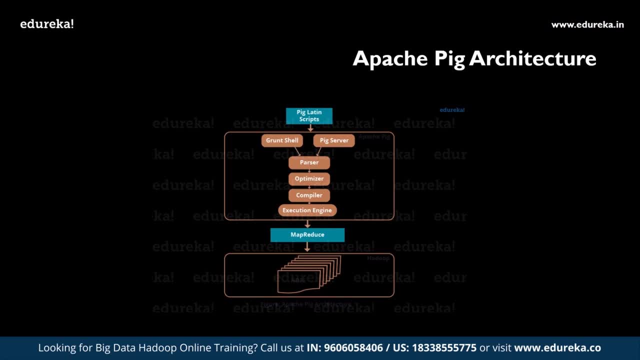 there are various components in Apache PIC framework. Let us look at the major components. Firstly, the parser. Initially, the PIC scripts are handled by the parser. It checks the syntax of the script, does type checking and other miscellaneous checks. The output of the PIC script. 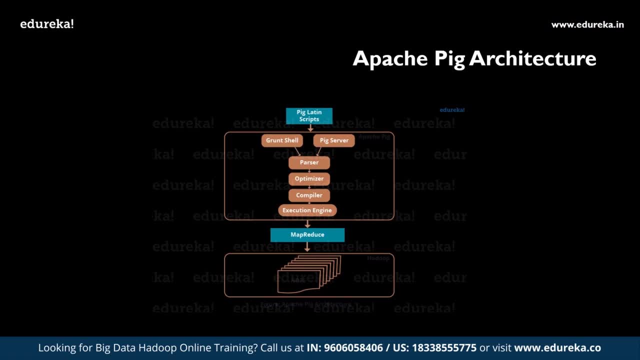 in the parser will be a DAG, which is directed acyclic graph, which represents the PIC Latin statements and logical operators. In directed acyclic graphs, the logical operators of the scripts are represented as the nodes and data flows are represented as edges. And next the optimizer. 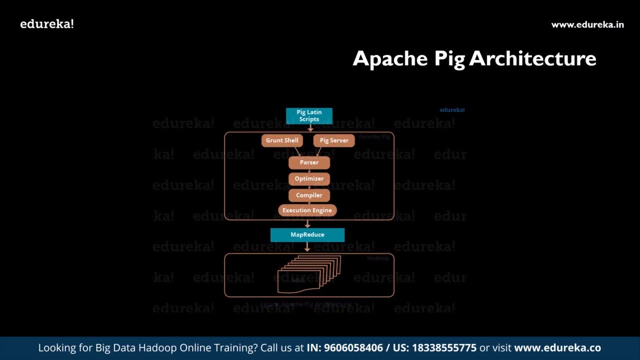 The logical plan for directed acyclic graphs is passed to the logical optimizer. This carries out the logical optimization, such as projections and pushdowns. Next comes the compiler. The compiler is used to compile the optimized logical plan into the series of MapReduce jobs. 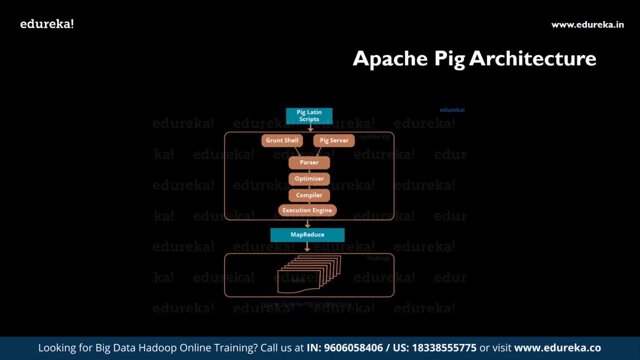 Followed by that, we have the execution engine. Finally, the MapReduce jobs are submitted to the Hadoop in a sorted order. Finally, these MapReduce jobs are executed on Hadoop, producing the desired results. So this was a basic explanation. 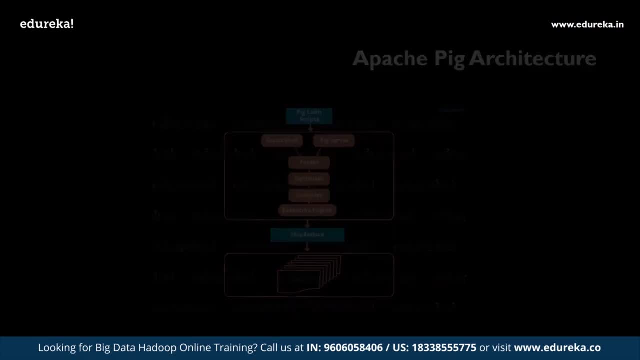 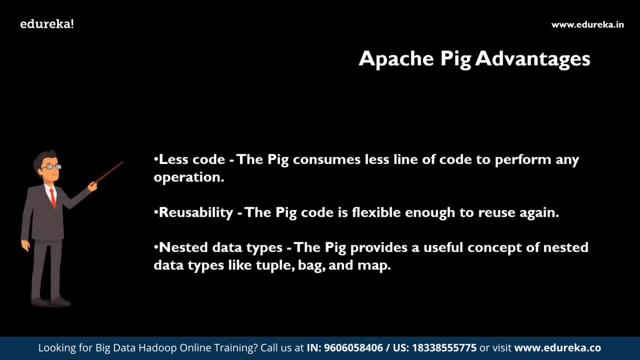 based on Apache PIC architecture. Now, moving ahead, we shall understand the major advantages of Apache PIC. So some of the major advantages of Apache PIC are: less code: The PIC consumes less than a line of code to perform any operation, So this reduces the number of lines. 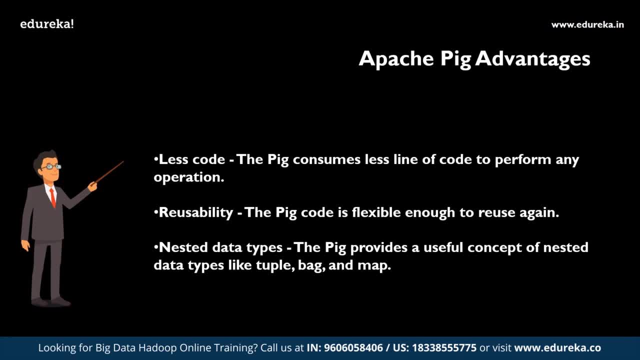 included in the code, Followed by that code reusability. The PIC code is so flexible enough to reuse it again. You can basically write the PIC script into a file and access the file whenever you need it. So, followed by that. 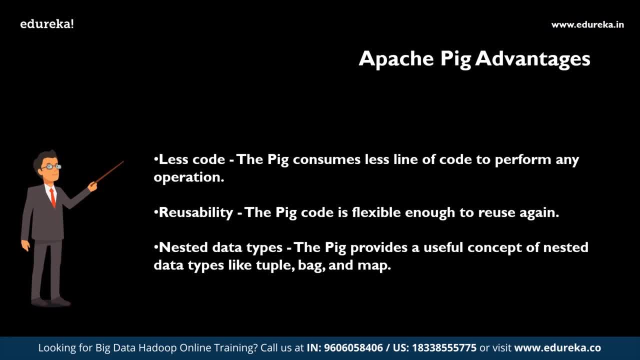 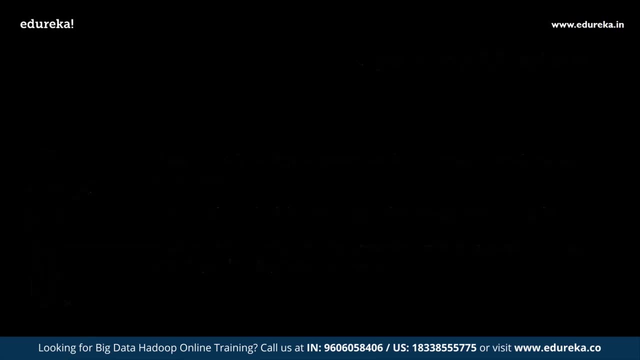 the next important advantage of Apache PIC is the nested data types. The PIC provides a useful concept of nesting data types like tuple, bag and map. So these were the few important advantages of Apache PIC. Now we shall move ahead into the next topic. 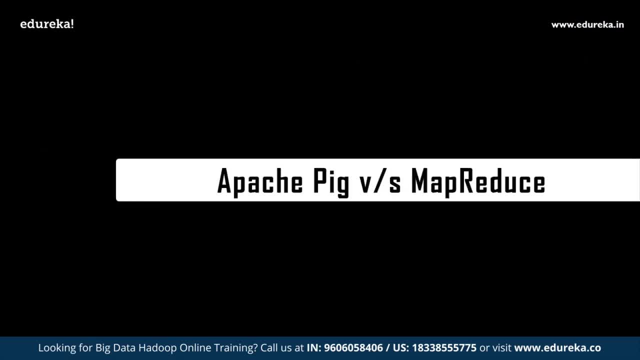 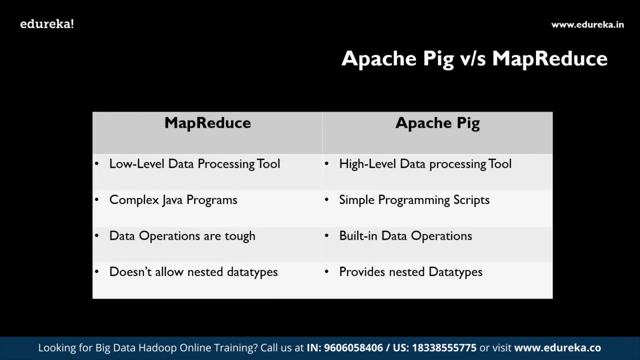 which is about the differences between Apache PIC and Apache MapReduce. So there are basically four differences between Apache PIC and Apache MapReduce. So first up, we will begin with MapReduce. In MapReduce we have low-level data processing. 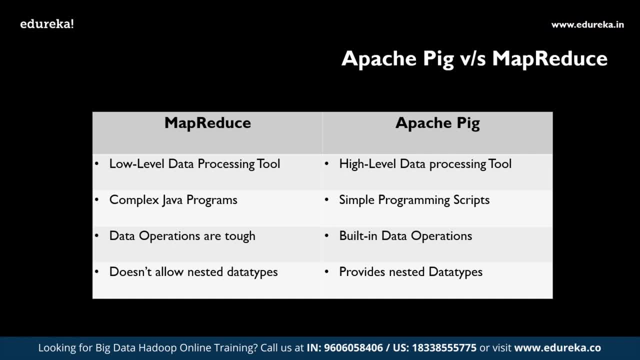 When it comes to Apache PIC, it is considered as a high-level data processing tool. Followed by that, the next important difference between MapReduce and Apache PIC is that we find complex Java programs when we are using MapReduce, But when we come into Apache PIC, 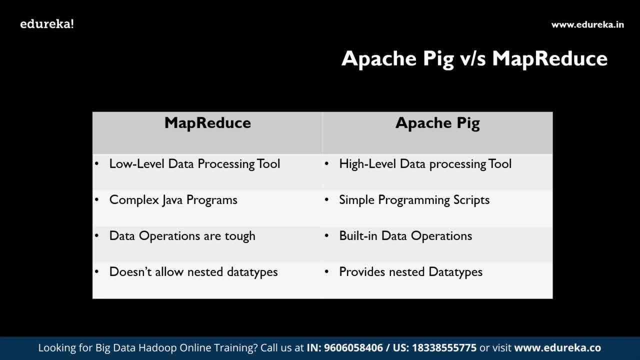 we have simple programming scripts which are shorter in code length and easily understandable. Followed by that, the third difference is the data operations are completely tough and complicated in MapReduce, But in Apache PIC you don't have to worry about those operations. 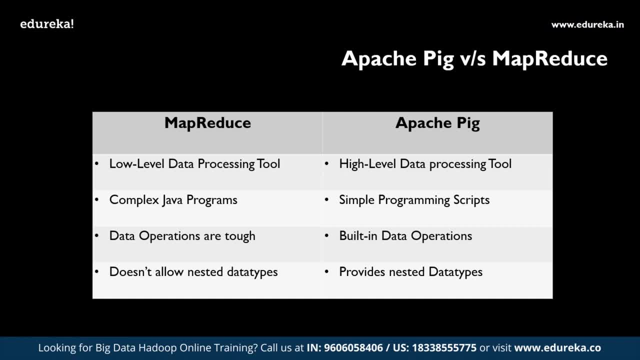 because they're already built in. Next and the last difference between MapReduce and Apache PIC is: Apache MapReduce does not allow nested data types, whereas Apache PIC allows nested data types. So these were the basic differences between Apache MapReduce and Apache PIC. 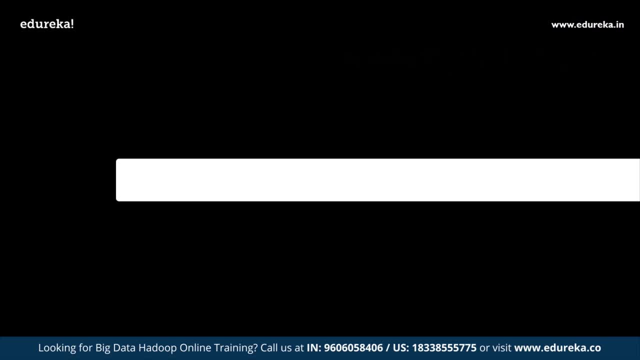 So the next topic is the PIC demo. Here we will understand all the basic commands in Apache PIC and the basic functionalities which are available in PIC. Now, without further ado, let's quickly begin with our demo for today's session. Now we have come back to our cloud era. 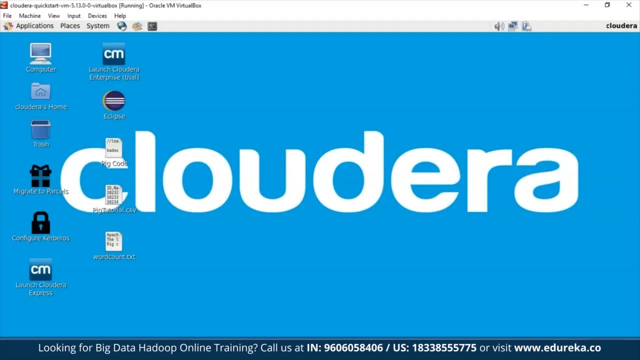 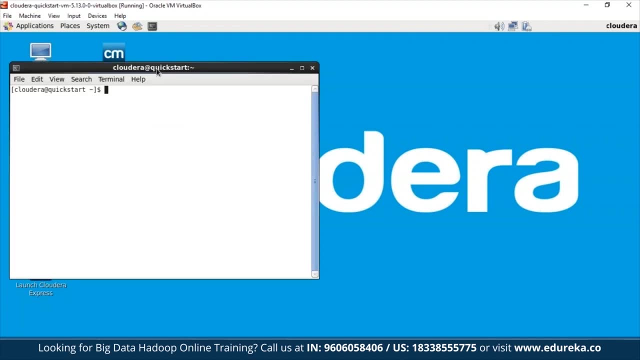 that we have installed into our local system. Now let's start PIC. As we have discussed before Apache, PIC can be executed in two modes. They are the local mode and the MapReduce mode. Firstly, we shall execute an example based on local mode. 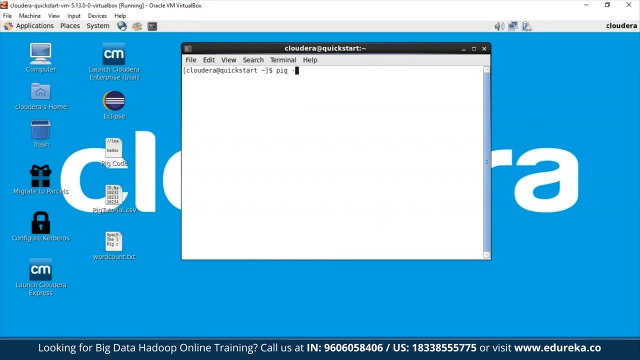 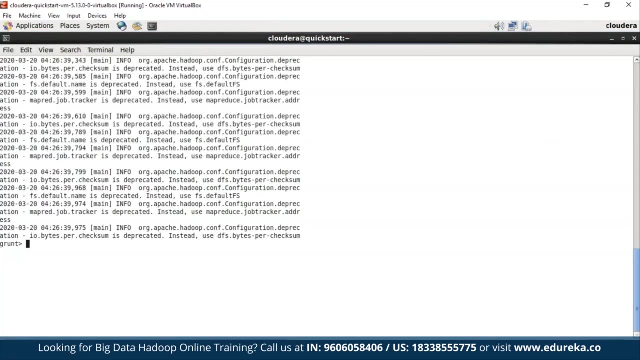 To start PIC in local mode, you need to type in the command PIC, hyphen x, space, local Firing. this command will enable PIC in local mode. As you can see, the command is getting decrypted. Now you can see that it has successfully started the grand shell. 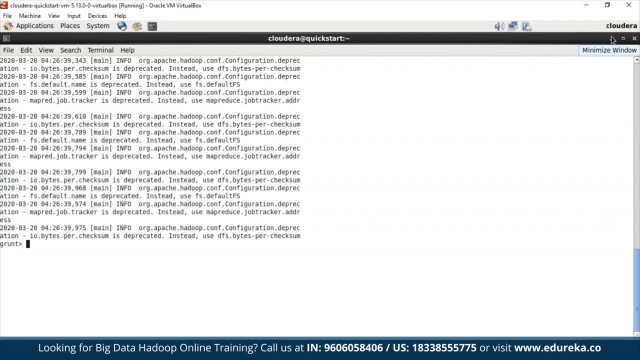 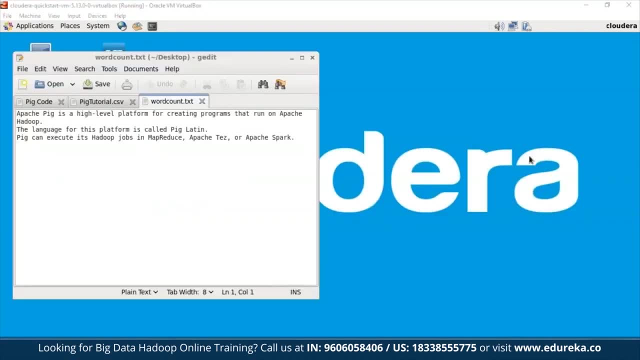 in local mode. Now, what are we going to execute? We are going to execute a very simple word count program. For this particular word count example, I have considered a basic text, that is, the definition of Apache PIC, which happens to be. 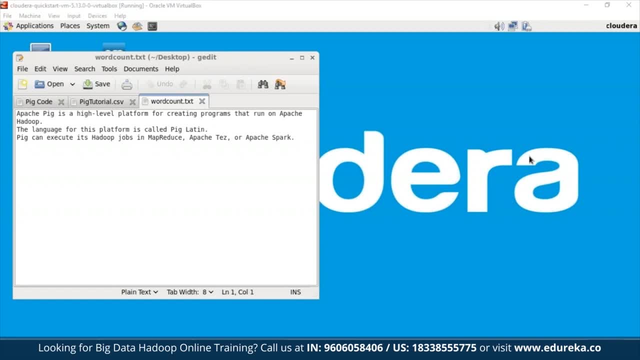 Apache PIC is a high-level platform for creating programs that run on Apache Hadoop. The language for this particular platform is called PIC- Latin PIC can execute its Hadoop jobs in MapReduce, Apache Test and Apache Spark, So we will consider this particular paragraph. 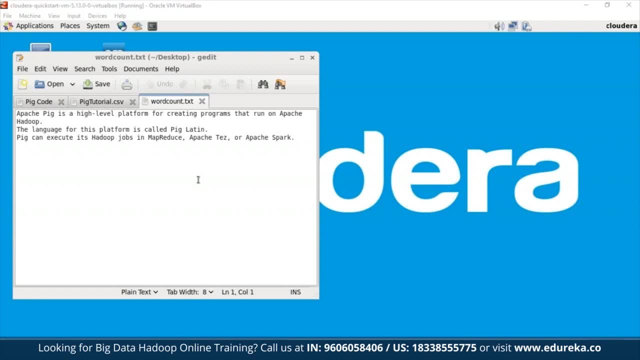 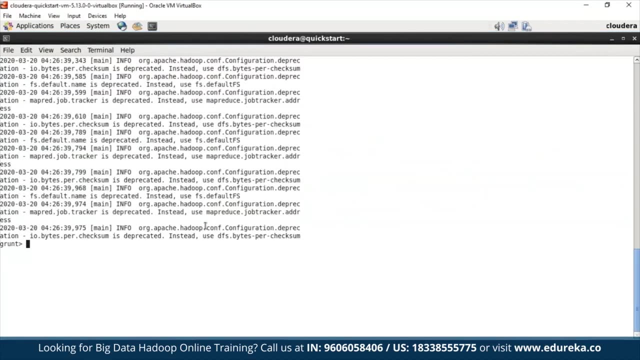 and we will also count the number of words which are included in this particular paragraph. Now let's quickly go back to our terminal and execute our program. So now we have come back to our terminal, Let's clear it using the command control plus L. 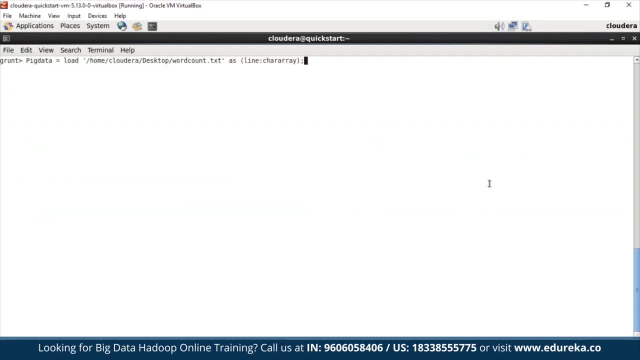 Now let's quickly start up typing our commands. So, as discussed before, we are going to execute this particular program in local mode. So here we are not loading the data into HDFS. Instead, we are considering the local location. 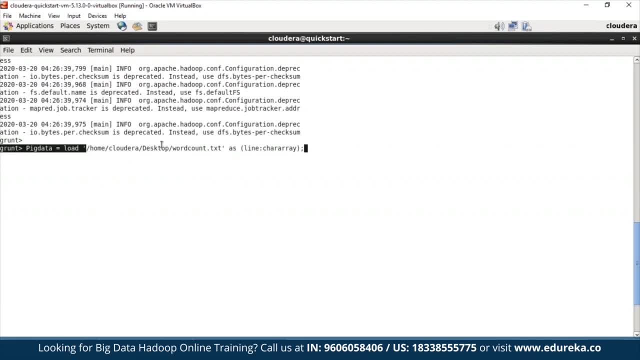 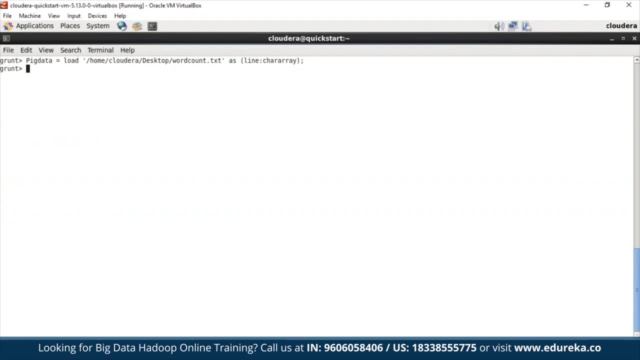 which is the local location that is home cloud at our desktop word count. Now we are going to run this command and see the output. So the data has successfully loaded. Now we'll execute the next command. So now we are going to tokenize each. 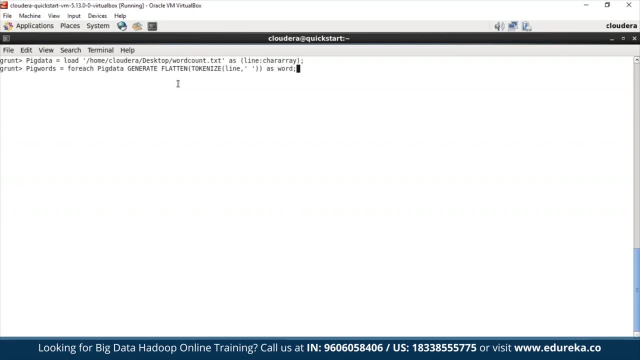 and every single word in this particular paragraph, and we'll be considering each and every word as a single word and we are going to separate each and every word by using a space. Now let's fire up this command and see the output. Yeah, the command just got executed. 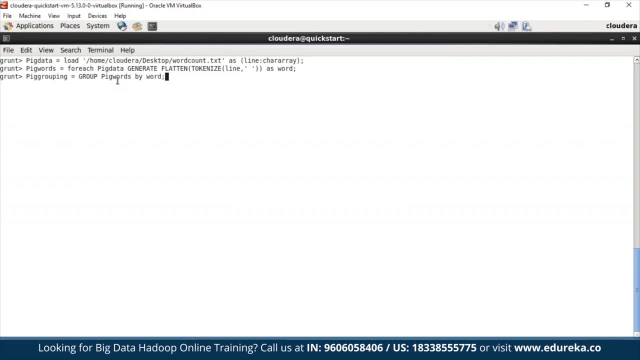 or the script just got executed. Now in the next script, we are going to group the words according to their occurrence. Yeah, even that is done. Now the next script would help us to count the number of words which have been repeated. 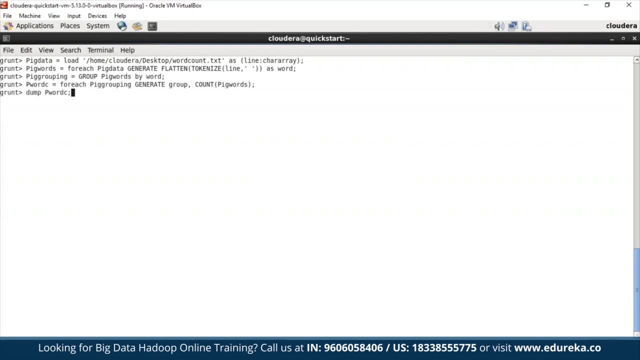 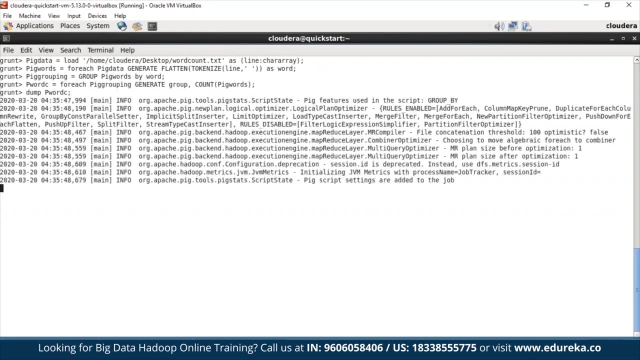 So even that is done. Now the last script would be dumping the output which is stored in pWordC, which is big word count. Now let's enter the command and see the output. You can see some MapReduce jobs that are getting executed, and there you go. 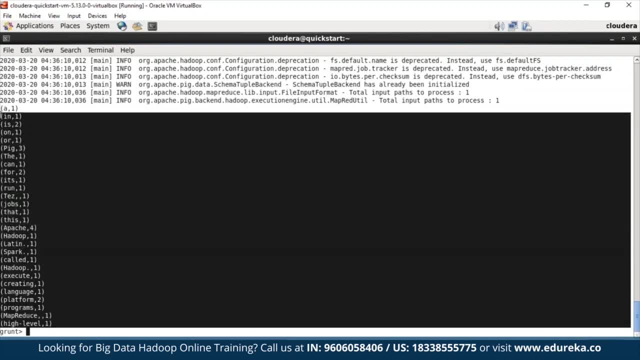 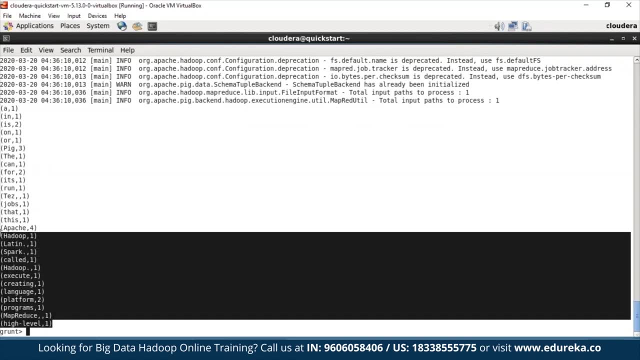 We have our output, So the words are a, n, on for its days: Hadoop, Apache and all those words, and along with them we also have the number of repetitions of each and every word. For example, we have Hadoop. 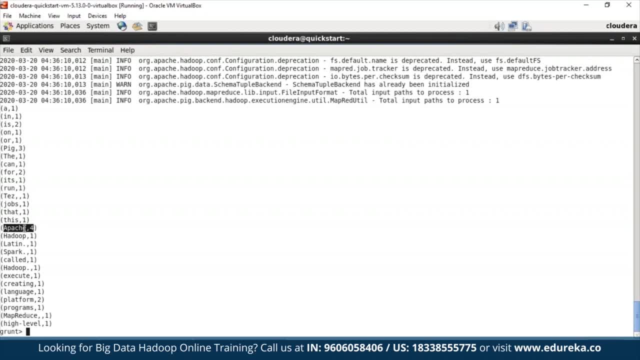 which is repeated one time, and the word Apache is repeated for four times, and so on. So with this, now let us move ahead and execute some examples based on Apache's Hadoop mode or MapReduce mode. Now let's close this terminal and open a new one. 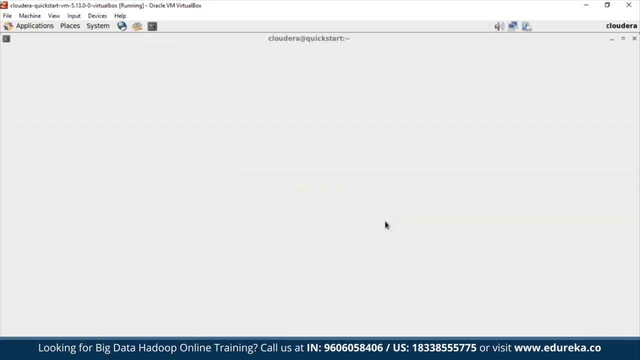 and let's begin executing Hadoop in MapReduce mode. As discussed before, Apache PIC can be executed in both local mode and MapReduce mode. We have already executed some examples based on local mode. Now we should execute some examples based on MapReduce mode. 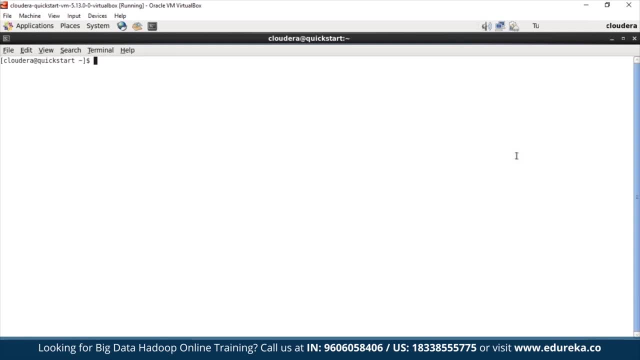 To do so, we will first load some local data into HDFS. So, using this command, I'll be loading my local data that has picked tutorialcsv into my HDFS and I'll name it as edureka-n, As you can see. 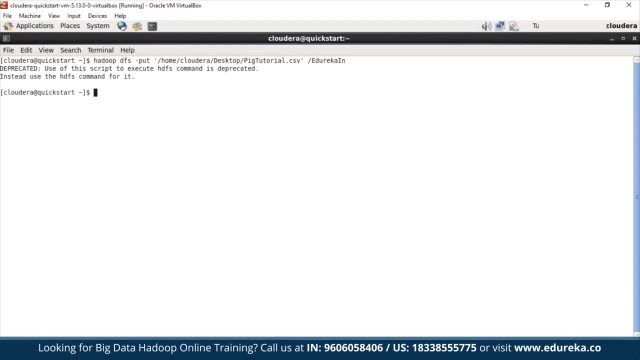 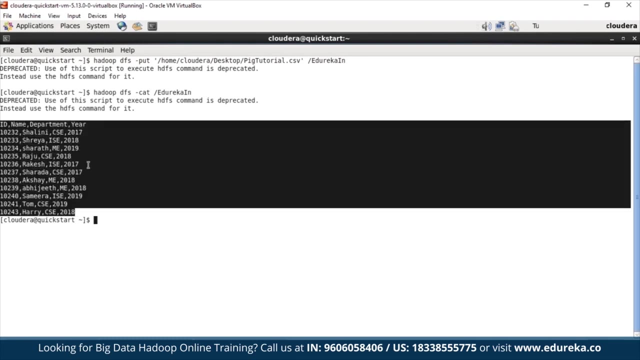 the command is getting deprecated and the data has been successfully loaded. Now let us use cat command and see what exactly is present in that particular data. As you can see, the command got deprecated and the data is a simple CSV file related to students. 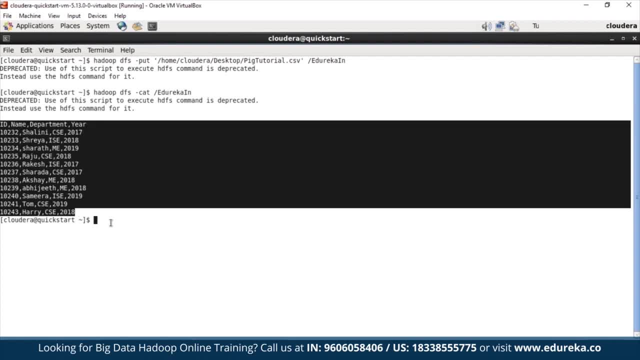 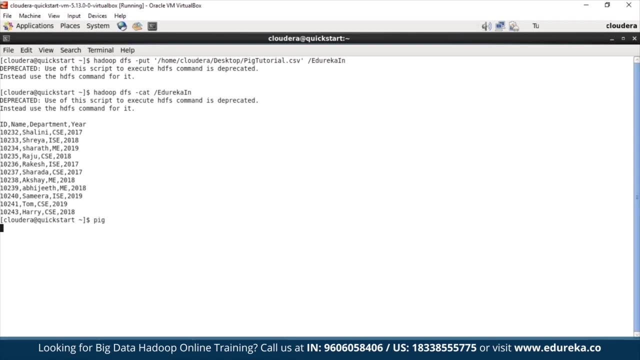 that has ID name, department and year. Now let's start PIC in MapReduce mode. To do so, we just need to type in pig and strike enter. There you go. We have successfully started PIC in MapReduce mode. Now let's execute some commands. 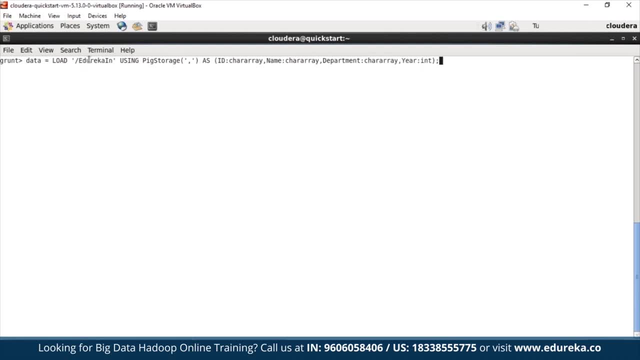 So, using this command, we will be loading edurekan, that is, the data, the CSV file which we have discussed before, using PIC storage as comma separated file, and the schema for the data will be ID as character array, name as character array. 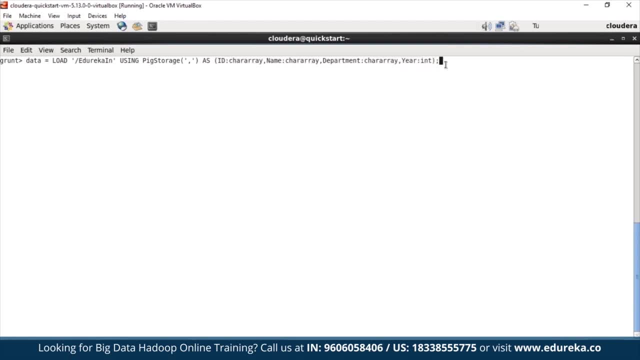 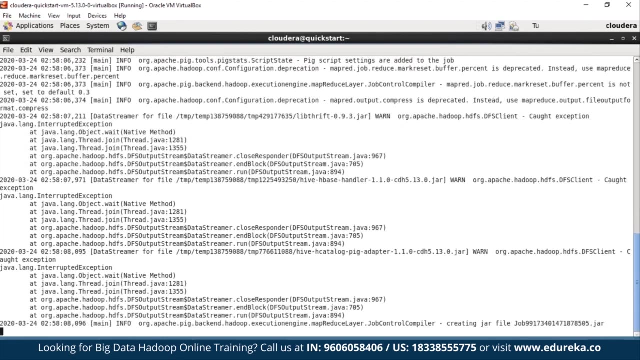 department as character array and year as integer array. Now let's strike an enter and see the output. There you go. The data has been successfully loaded now. Now let's use dump command to see the data, what we have loaded. So there you go. 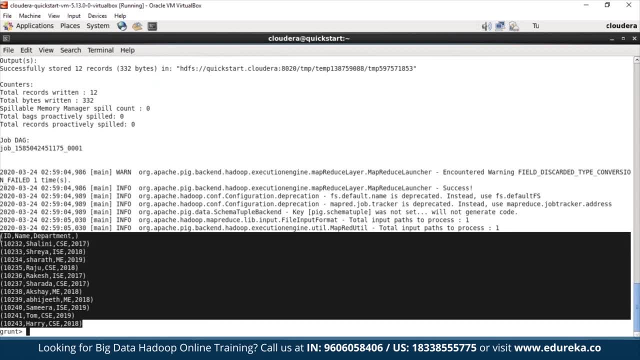 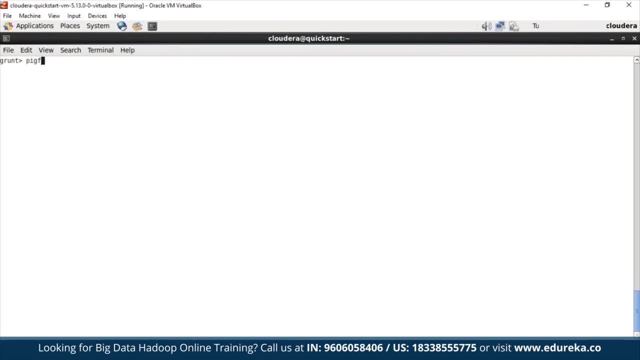 The data has been successfully dumped, So this was the data which we have loaded. Now let's move further and execute few more commands. Now we shall use: for each command and for each data present in our data file, we will generate ID, name and department. 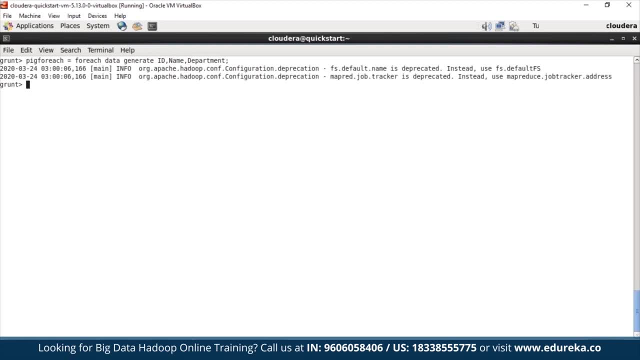 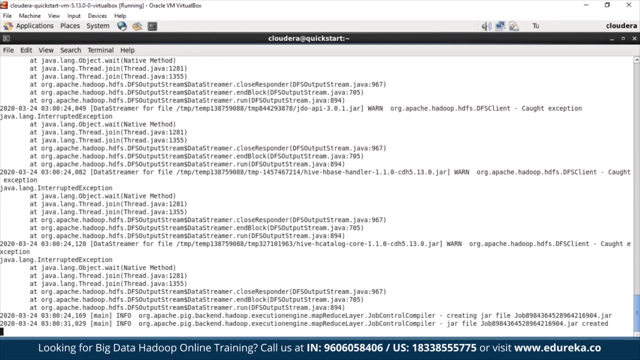 There you go. The command got successfully executed. Now let's dump the data using dump command. So PIC for each is our variable that stores the data. Now let's type in semicolon and enter. So there you go. 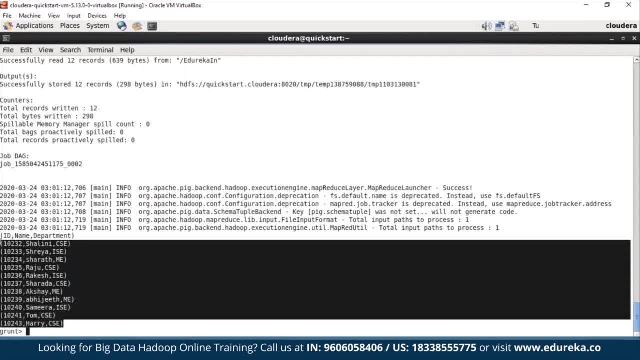 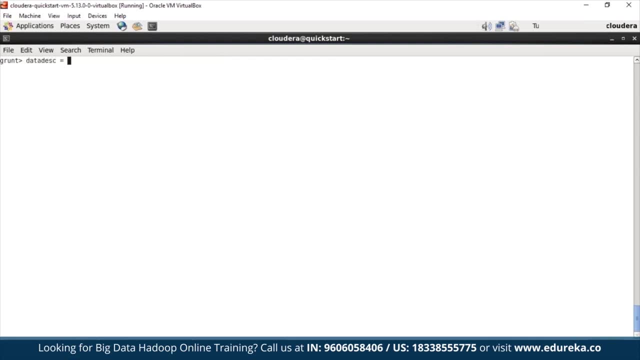 The for each command has been successfully executed and we have generated ID, name and department. Now we shall execute few more examples. Now we shall use descending operator to arrange the data in the form of descending order of ID. So it's been executed. 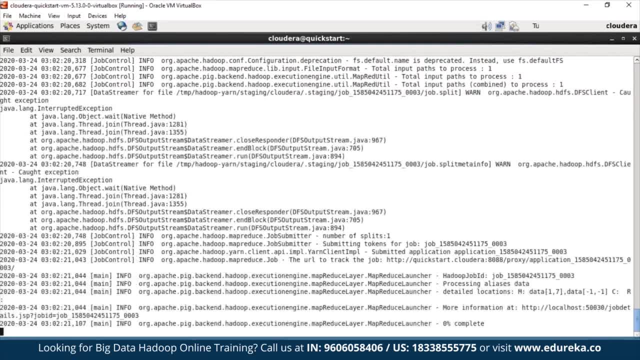 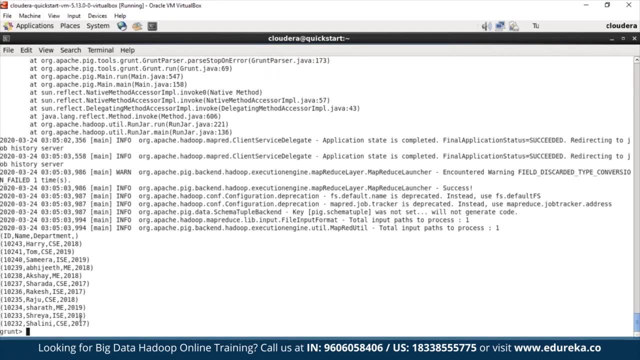 Now let's dump the data and see the output. There you go. We have successfully executed the dump command and the IDs are arranged in the descending order. now, as you can see it Now, this is how the order by descending function works. 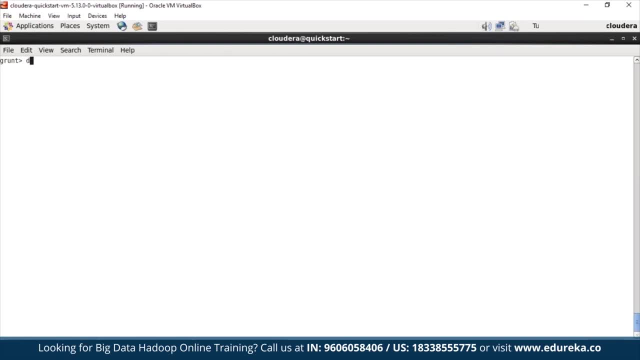 Now let's move ahead and execute one last command. As you can see, here we are using filter operation. We are going to filter the students based on the department, where department is equals to CSE. So executing this command will give us the students. 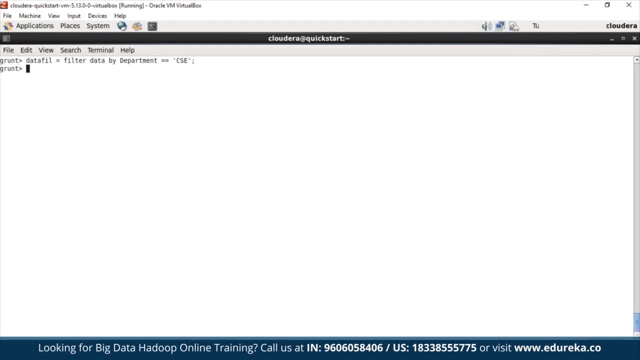 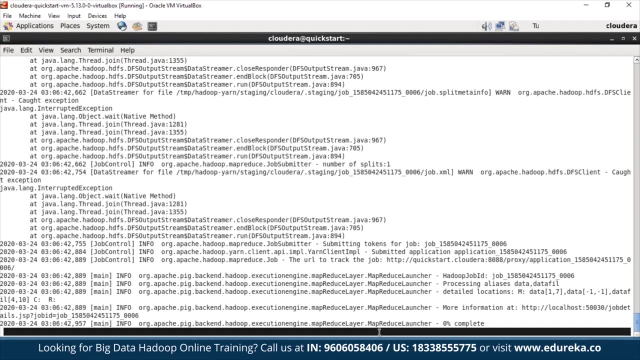 which are inside the department CSE. Now the command got executed. Now let's dump the data using dump command. So there you go. You can see some commands getting deprecated Here. you can see the MapReduce shops getting executed.